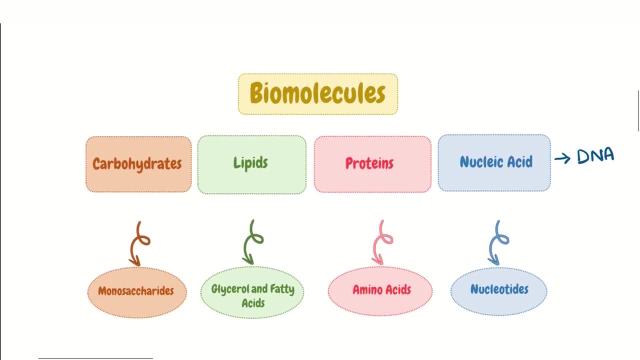 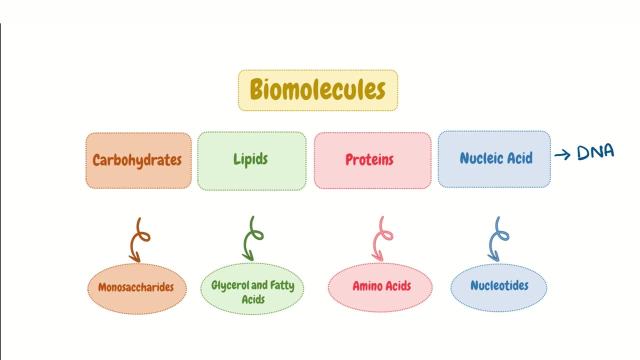 monomers, Like like monosaccharides, build carbohydrates or carbs, Glycerol and fatty acids make lipids, and that of proteins are amino acids. And what about the fourth one? What are the building blocks of our DNA? So here jumps in the topic of the 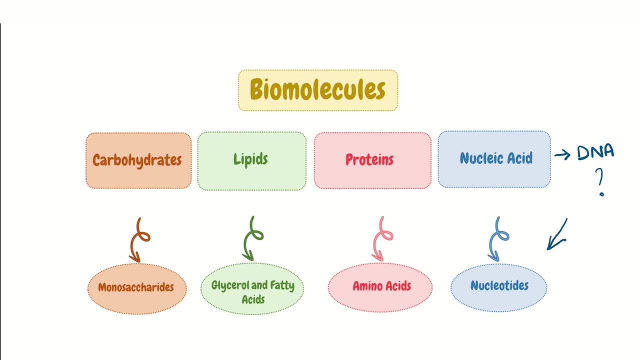 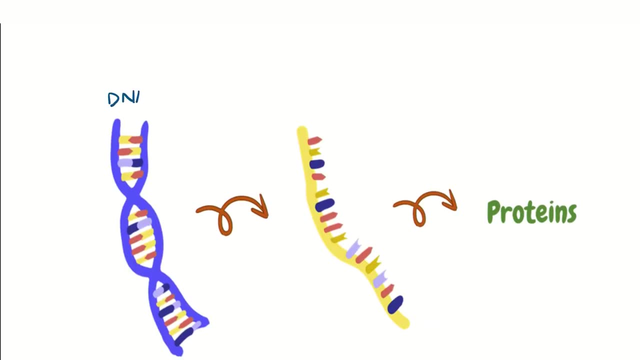 day Nucleotides. Yes, nucleotides are the building blocks of nucleic acids. Now our DNA is converted into RNA through the process of transcription, And RNA converts to protein through translation. So nucleotides are essentials for all cells. 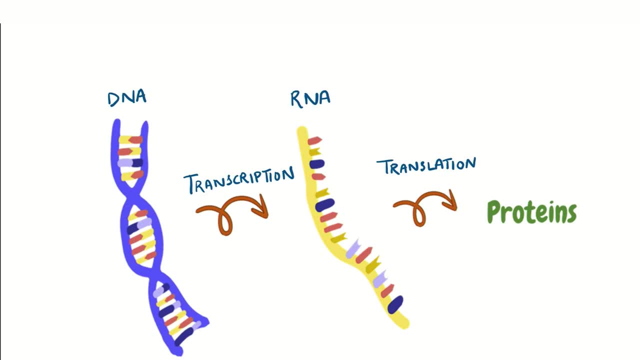 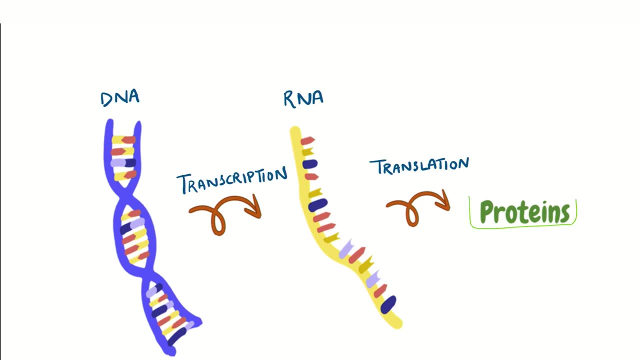 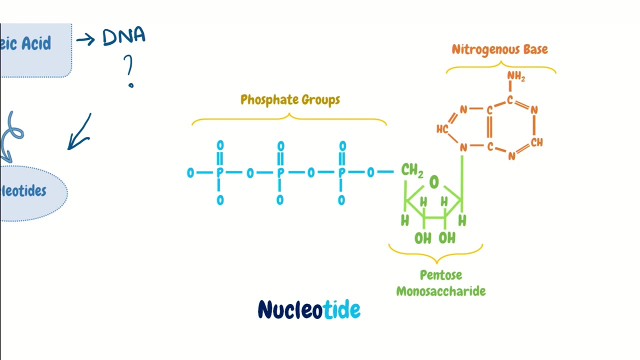 Without them, neither deoxyribonucleic acid or DNA, nor the ribonucleic acid or RNA can be produced, And therefore proteins cannot be synthesized, nor can cell proliferate. So now, nucleotides are composed of three main components: a nitrogenous base, like as you can see here. 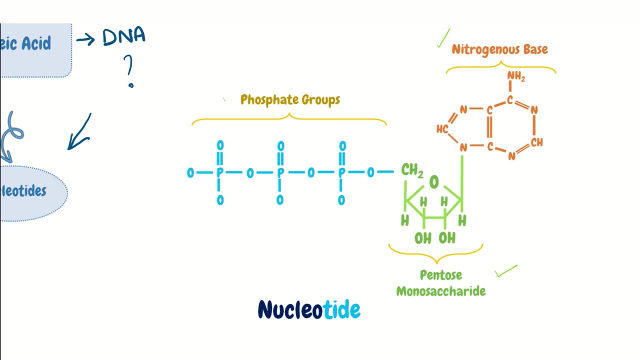 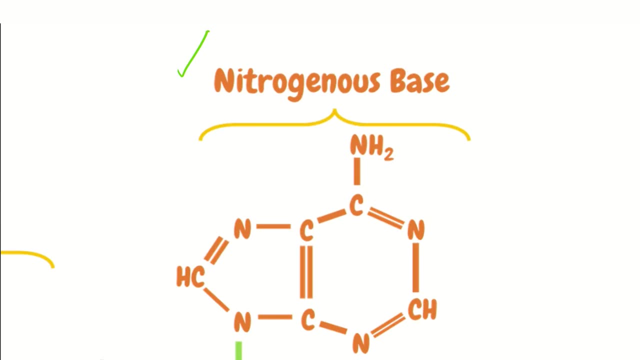 a pentose sugar and two to three phosphate groups. So now, first we'll talk about nitrogenous base. So nitrogenous base- name giving you a hint that nitrogen is a must. Now, they belong to two different families of compounds: The Purines, 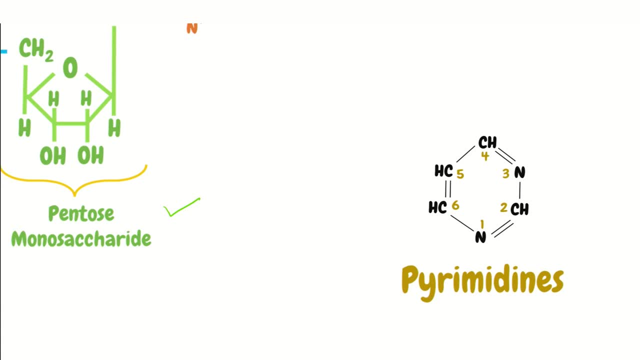 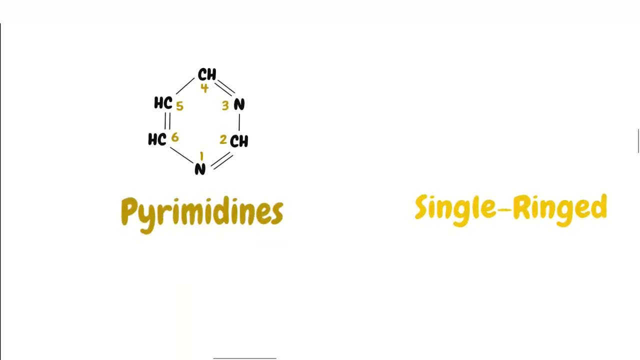 and the Pyramidines. Purines are double ring structures, whereas Pyramidines are single ring structures, A point worth noticing, as this is going to help you remember their structures. Well, I used to remember this in my school time by the fact that the one 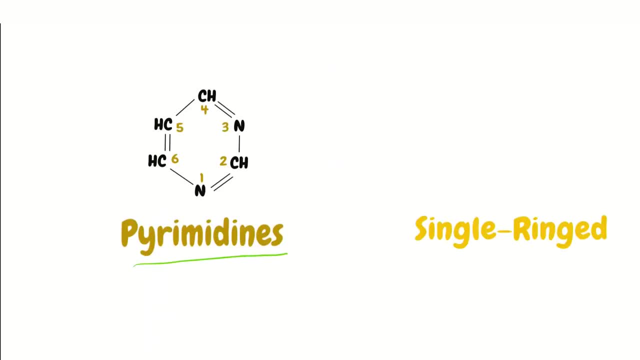 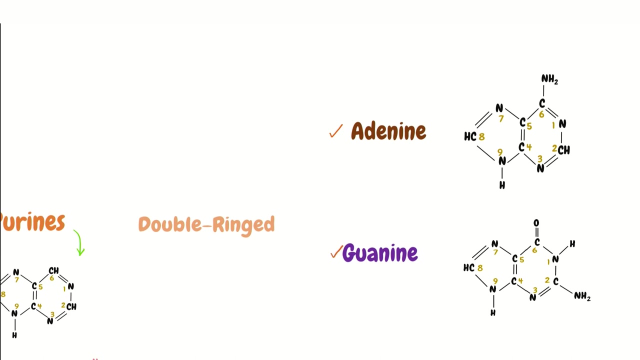 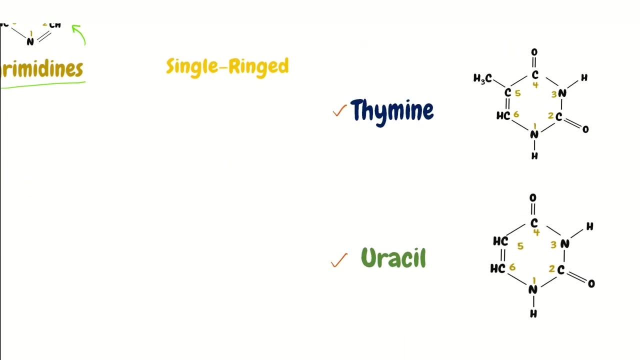 with the longer name. this one has a smaller structure And the one with the shorter name has a bigger structure. Now there are five common nitrogenous bases: Adenine, Guanine, Cytosine, Thiamine and Uracil. These are often denoted with their initials.